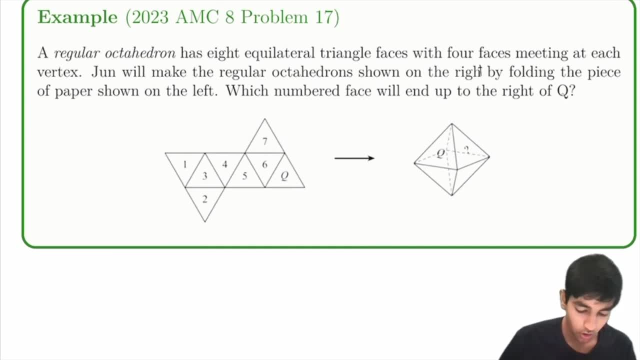 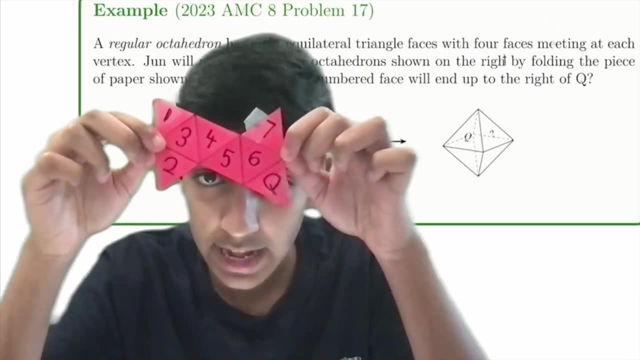 But the problem is, if we just got a bunch of triangles like, it's hard to figure out how this will actually fold, Rather than doing this in 2D, let's do it in 3D. So we've got our net over here, like that. 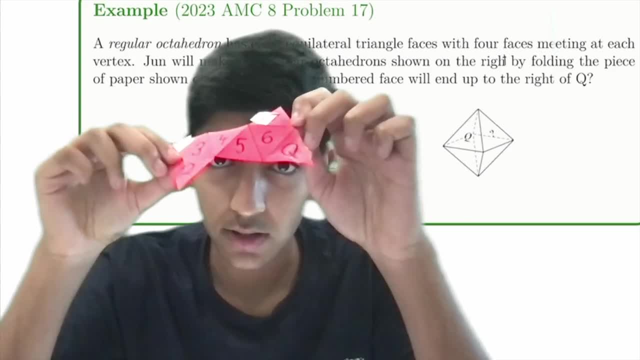 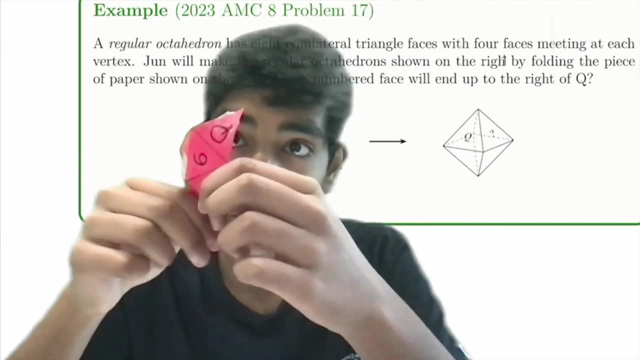 So what we can do is fold it along Q, because that's really the thing we're trying to focus on here. Let's rotate it upwards, like that, And then Let's do it like: move it like this, maybe notice that Q, or maybe the other way. 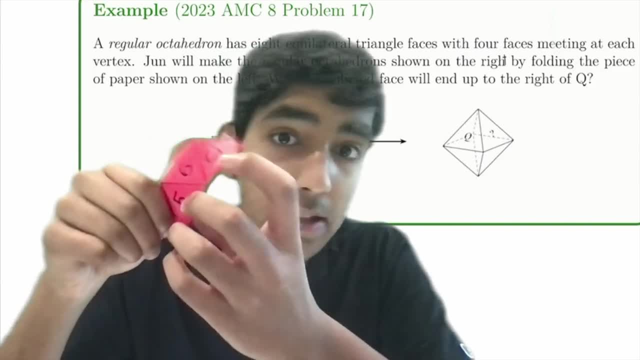 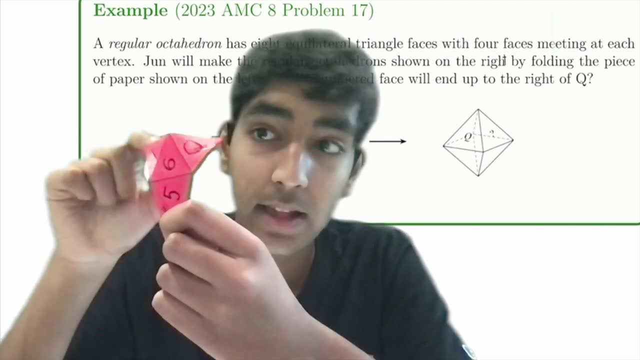 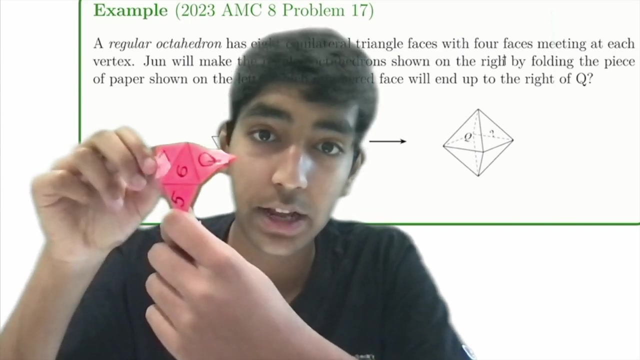 Yeah, like this. And now notice that Q is next to six on the six is on the left side of Q And then there's something else on the right side of Q and then seven all the way here is even next to six. So Q, six, seven over here. 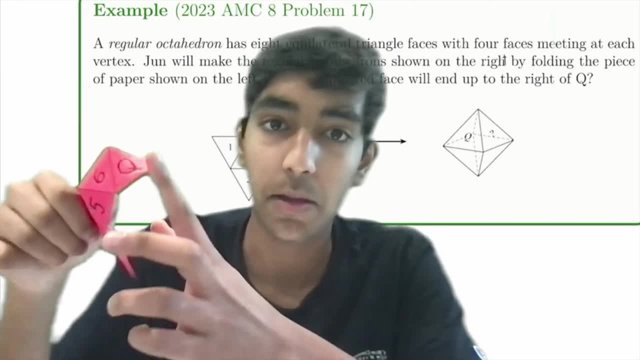 And then there's something in between here, which is basically what we're trying to find out in the problem right Cause there's Q, there's six on the left side, But we're trying to find out what's on the right side. this: 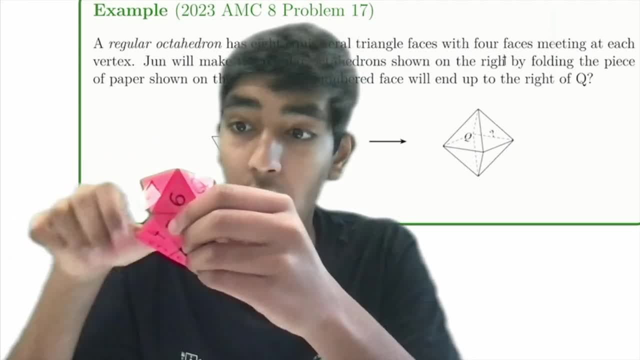 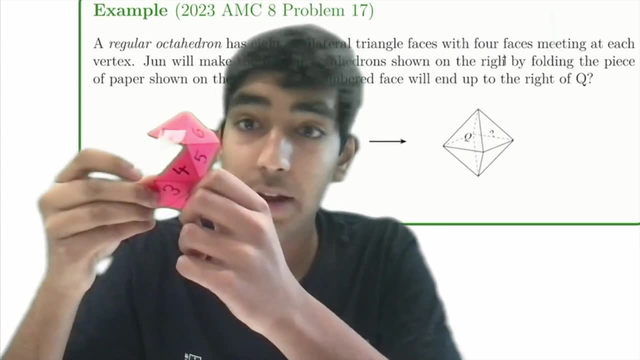 There's something missing here. So to find that out, let's just fold up what other things. So five will go right below six. It'll fold down like nicely, like that Now also we would have that four and seven will fold together. 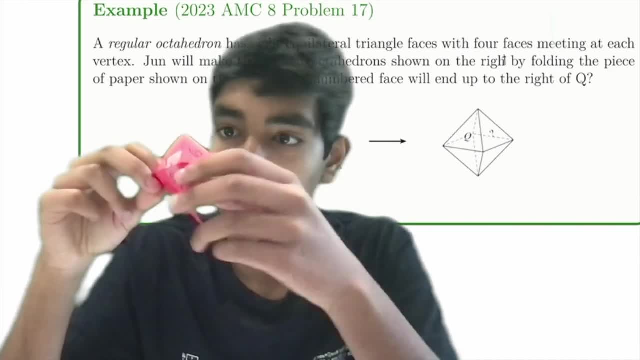 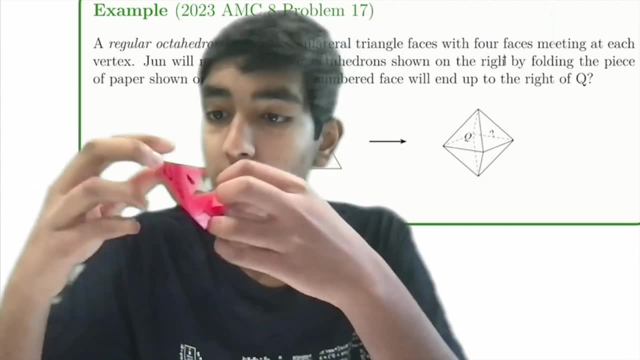 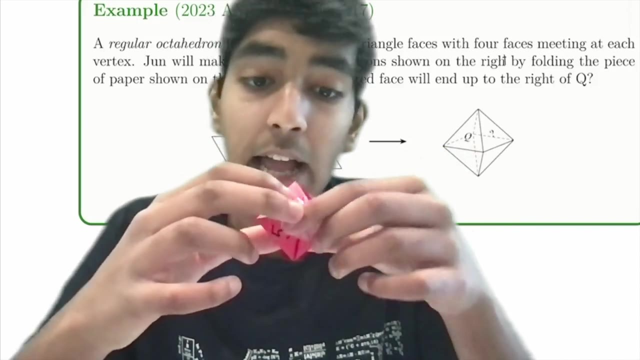 Let's fold that together. Boom, Four and seven are folded together. Now, looking at the back of it, we've got three, And then three, two and one. So let's fold two down here and one down here. So now that we have a 3d diagram, let's see how everything looks together. 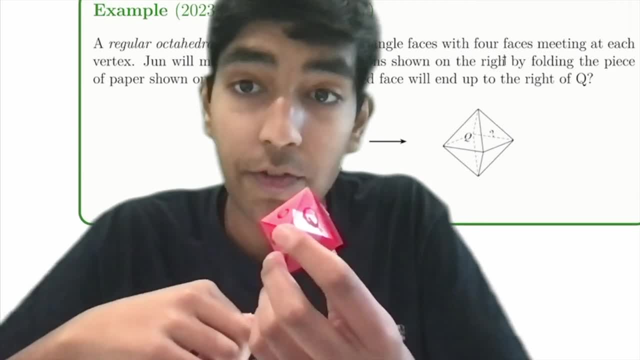 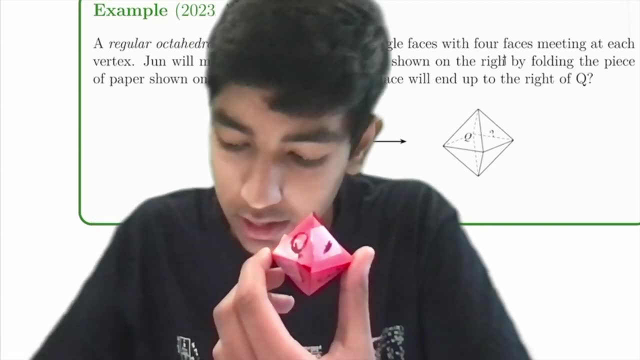 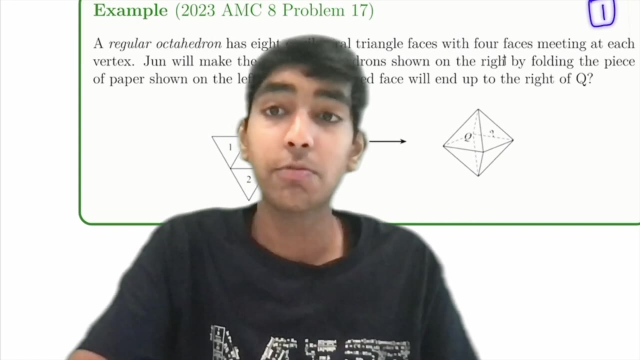 So we've got Q over here, and right on the left side of Q we've got six, but on the right side of Q, which is what the question is asking for, We've got one. Our answer is one: Okay, So let's see. how would we ever post this? 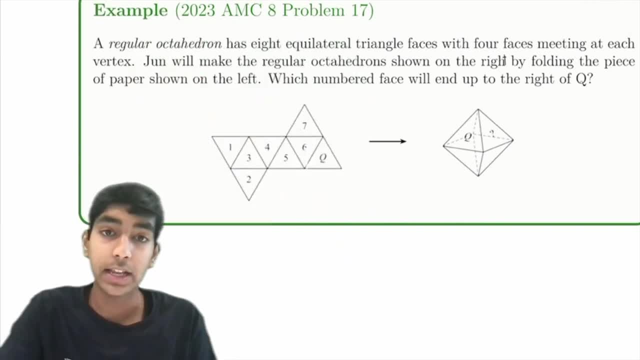 Problem if we had to, not if you could not use a 3d diagram, which, by the way, you can make in the real contest if you want it to. we've got Q here and then six will be right here next to Q.